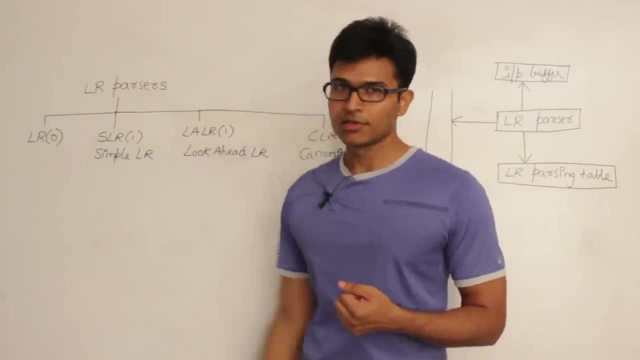 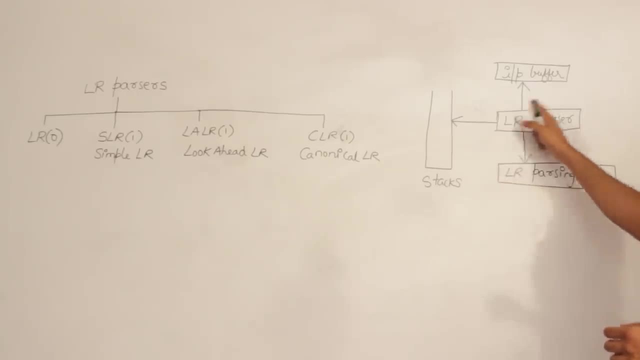 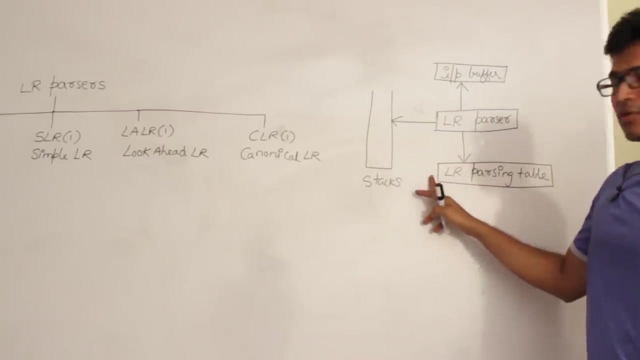 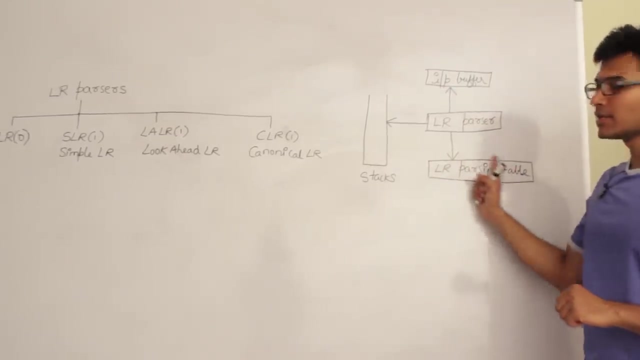 So this is the ascending order of their pass. So least powerful is LR0 and the most powerful is CLR1. And now, how does this LR parser work? is LR parser is an algorithm. And now this algorithm requires: one is input stack and other is LR parsing table and other is input buffer. So it is same as the bottom up parser, LL1.. In LL1, what was the parsing table? It was LL1 parsing table. right In LR, what is the parsing table? It is LR parsing table. 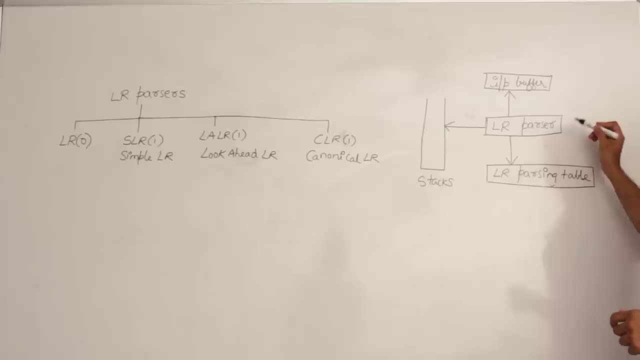 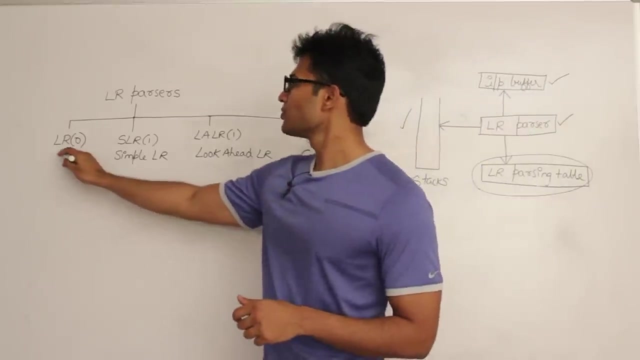 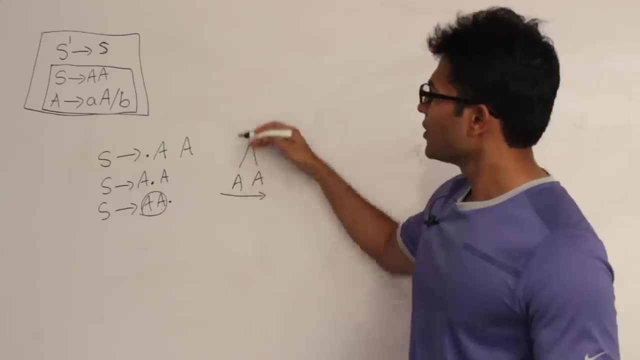 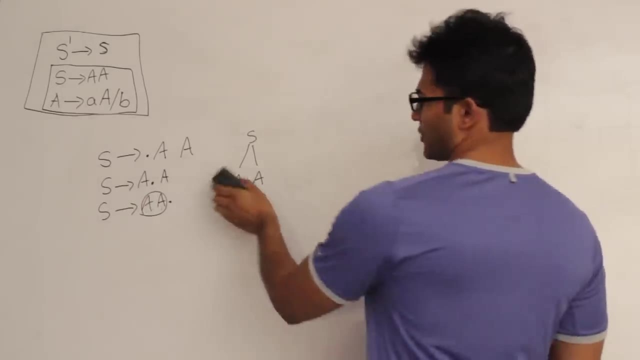 you see completely the right hand side, then we should reduce it in order to remember that we have seen everything in the right hand side. i am going to use this production right, so f0 cia is the production. the reason is: i have seen everything in the right hand side. now these l? r 0 items or 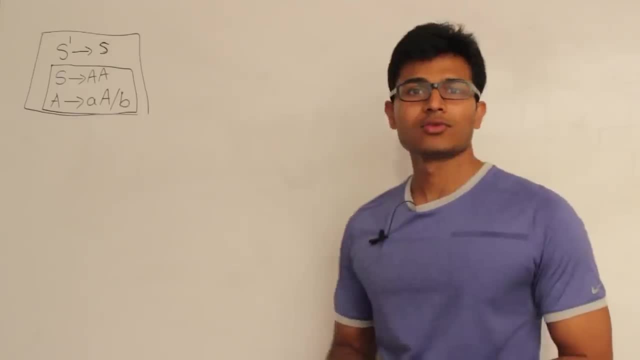 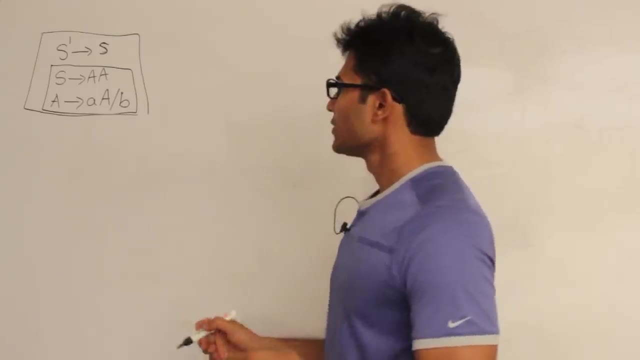 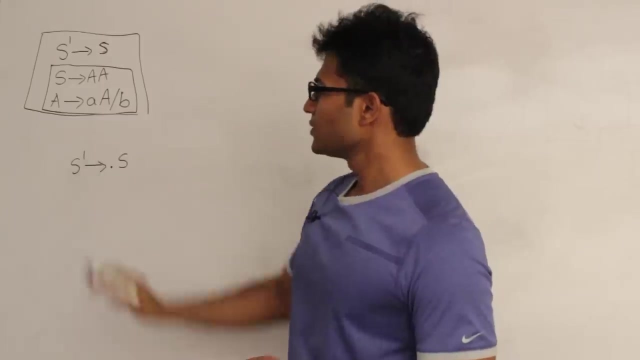 items are going to be helpful whenever you want to know that till what part we have seen the input and whether it is at the right time to reduce it or not. so now, first thing is s dash derives dot s. this is the starting point. now i have taken the l r 0 item for the first production. 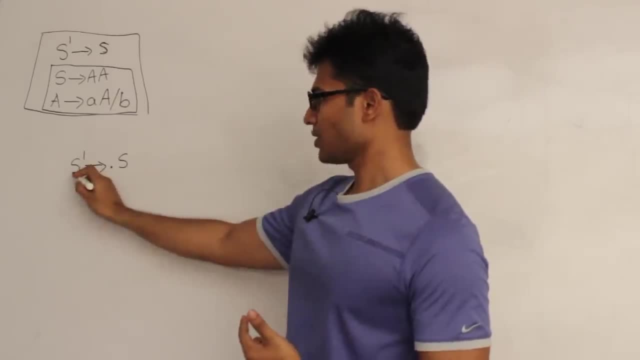 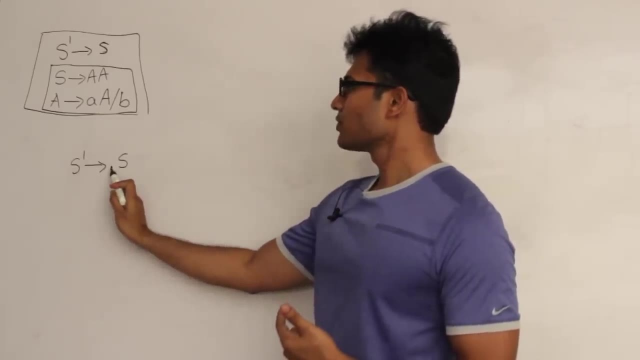 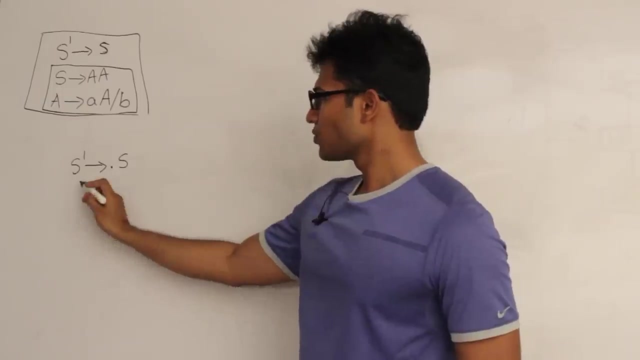 now i apply the closure. this is called the starting production and with dot i am going to apply the closure. closure is nothing, but whenever there is a dot to the left of a variable, you have to add all the productions of that variable with dot in the beginning. see, there is a dot to the left of the variable, so closure includes s, derives, dot, a, a. 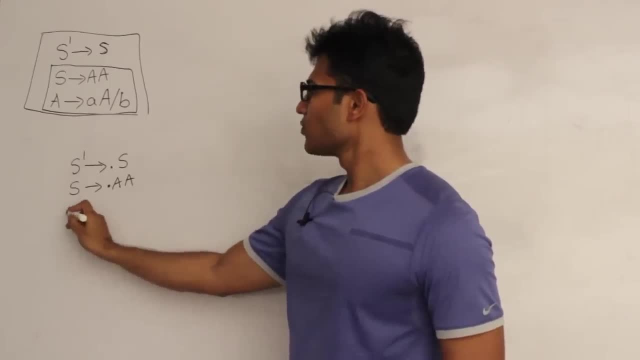 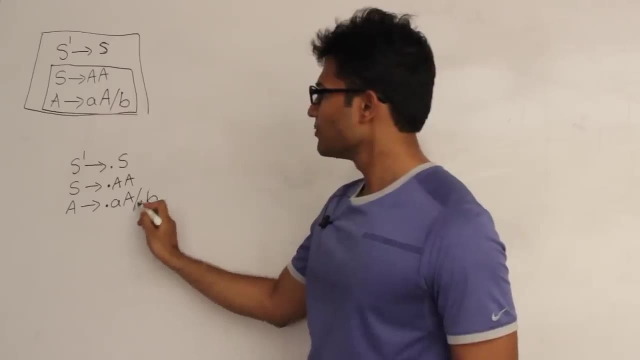 and again there is a dot to the left of a. therefore i have to again add the remaining productions. a derives dot a, a or dot b. it means that whenever you see a dot to the left of a variable, you are going to add all the productions with dot in the beginning. can i add any more? 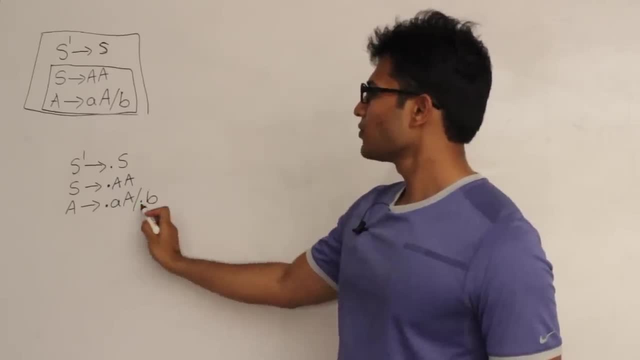 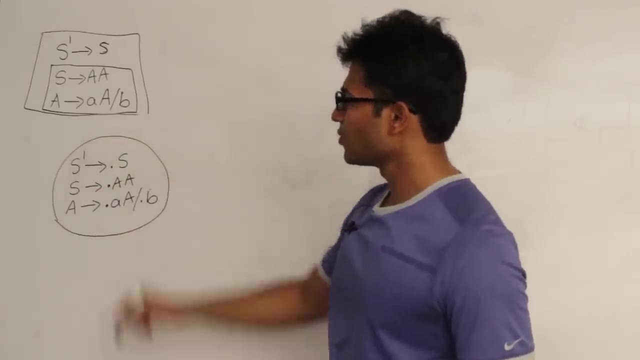 productions? no, because they are. there is a dot to the left of the terminals. therefore, you can stop here. this is the closure of s derives dot s. this is the closure of it. now. after that we have to do: go to go to means. it is simply like a dfa. 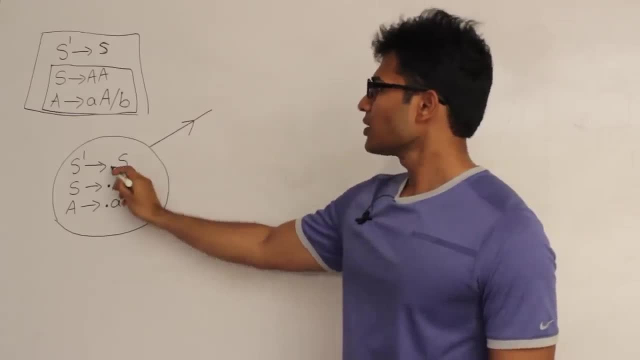 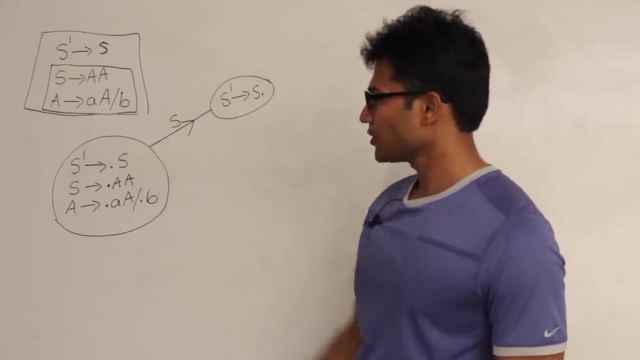 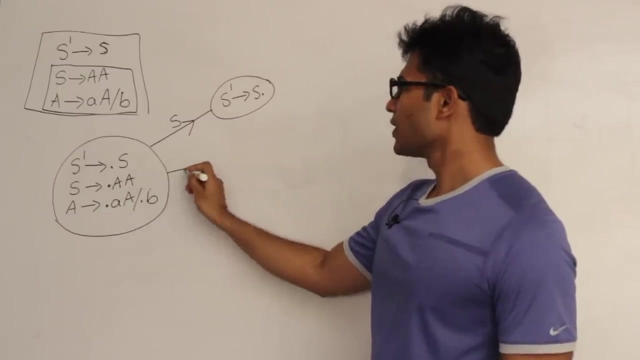 so, on this state, if there is any dot somewhere, if i move the dot over the next symbol, which means if i move this dot over the next symbol, what do i get? i get s dash derives s dot. i am just moving right of it, isn't it? now, if i look at this one, if i move the dot to left of a, to the right of a, 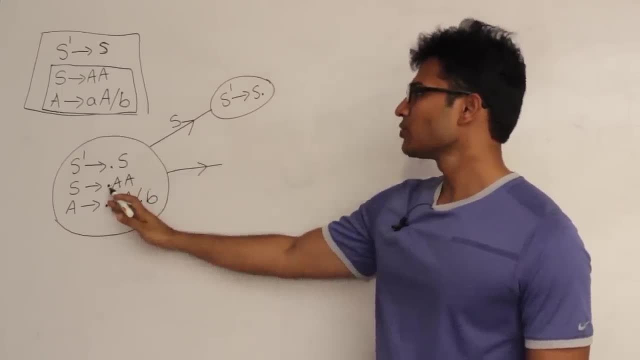 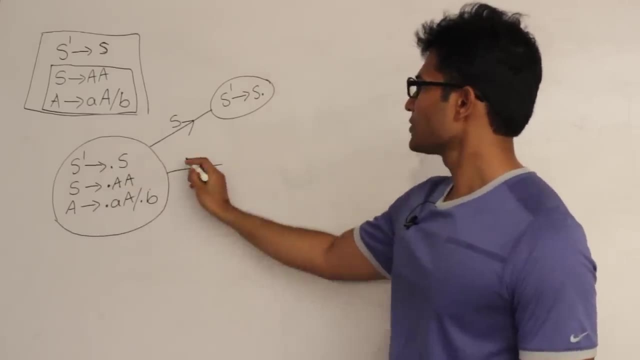 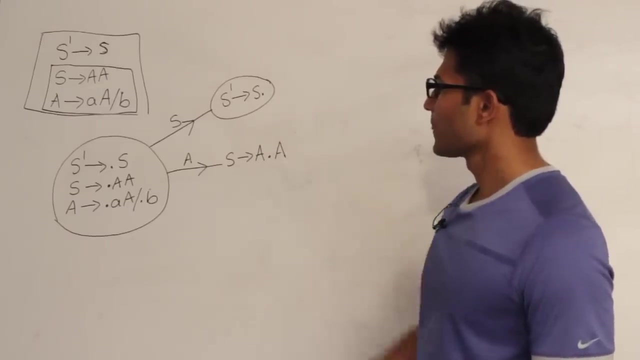 the dot is to the left of a. i am moving it to the right of a. it is also called as go to. this is a canonical collection of l r 0 items and now i am just moving it. s derives a dot a. now you have to apply closure whenever you apply go to. 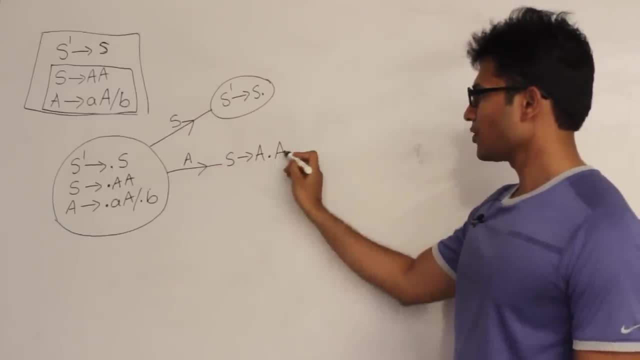 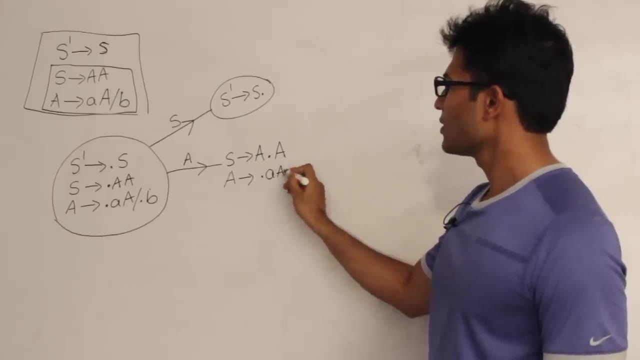 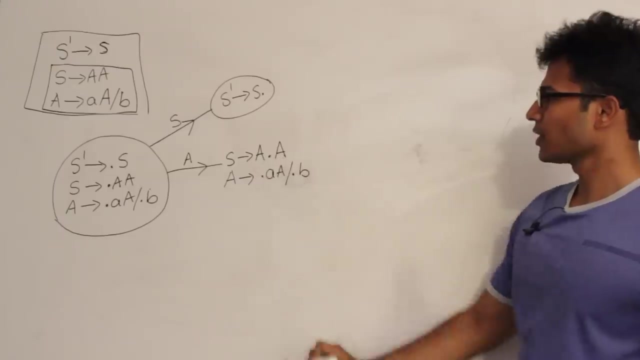 this go to is over. now you apply the closure. if i apply the closure, i get all the a productions with dot in the beginning. so what are all the a productions? a derives dot a, a or dot b. why did i add these two productions? because there is a dot to the beginning of a. okay, that is why i got this. 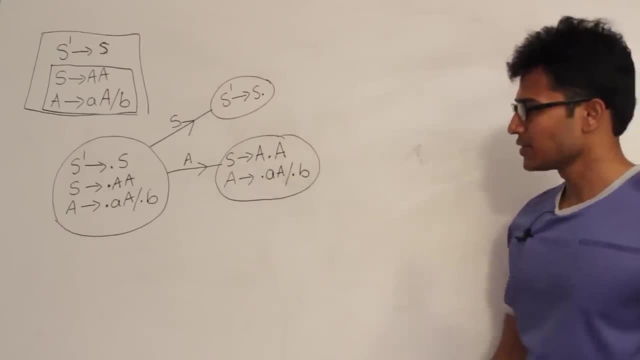 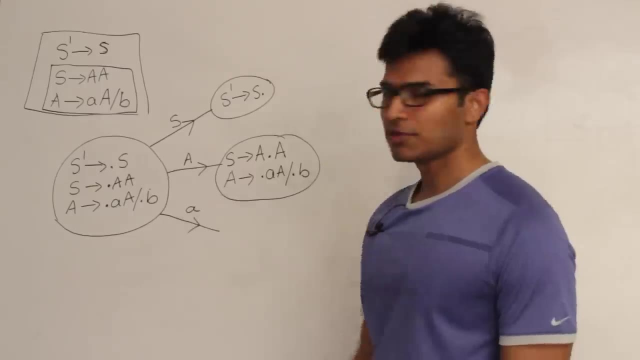 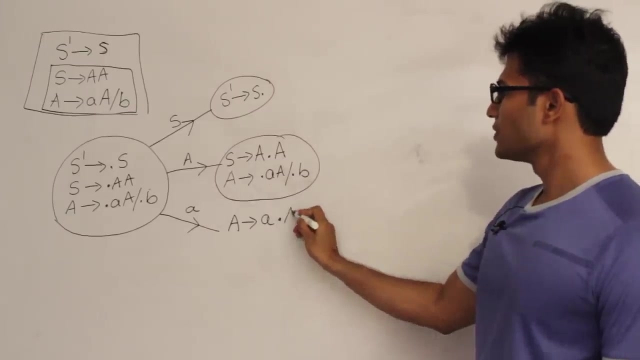 i don't get any more productions now. what are the other transitions? or what are the other go to items i have on small a? you can again go to one more state on small a. where do you go? a derives small a, dot, a, which is nothing, but i am moving a dot from the 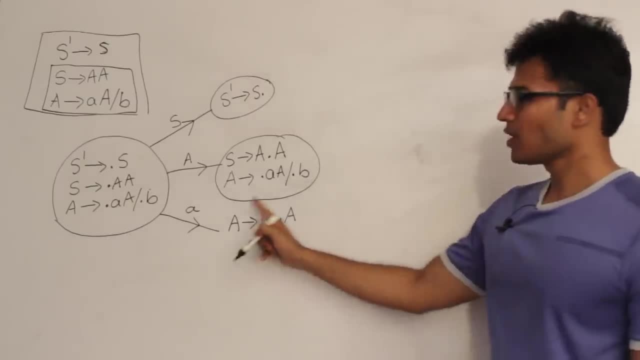 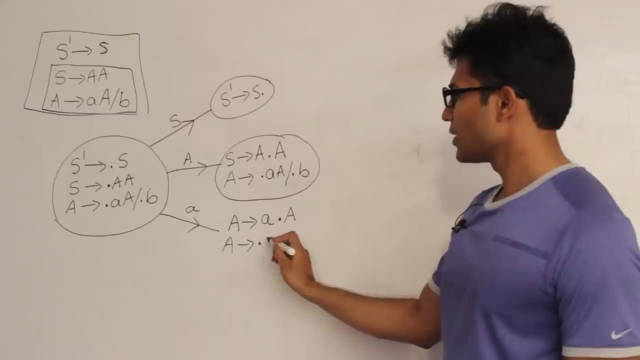 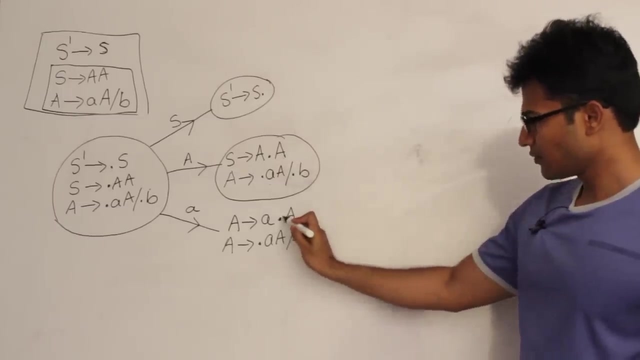 left of small a to the right of small a. okay, and now we have to apply the closure. if i apply the closure to this, what i get is a derives. if i am applying the closure, a derives, dot a, a or dot b. why did i get these two productions? because of this dot, this dot b before capital a. 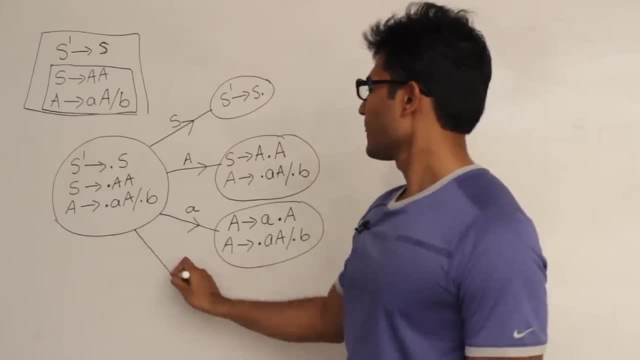 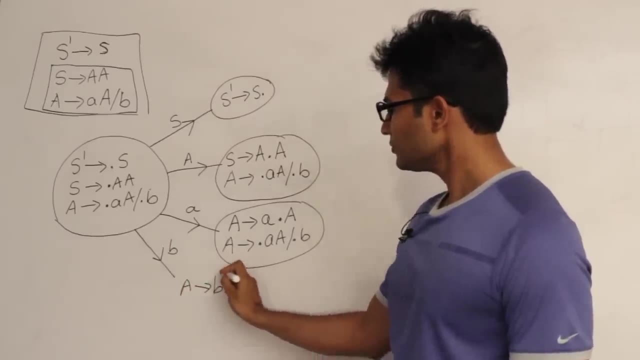 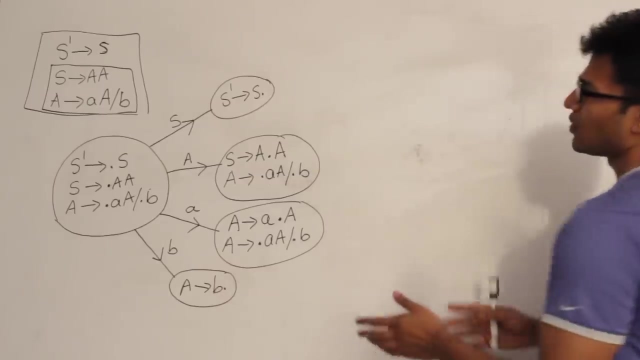 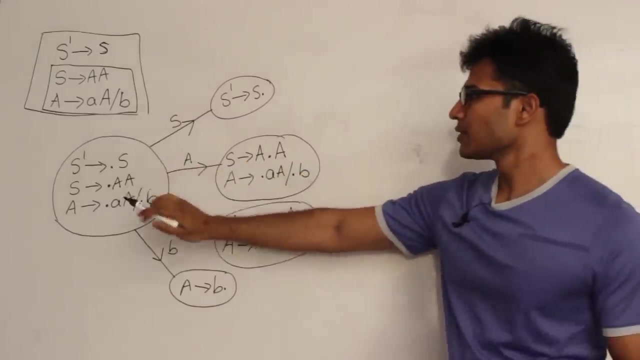 right and then b on b, i get a derives b dot. so what is the importance of this production? is this production is it is also called as final item. whenever dot is to the right, right hand side, rightmost side, it is also called as final item. okay, now this one is complete on s we have shown. 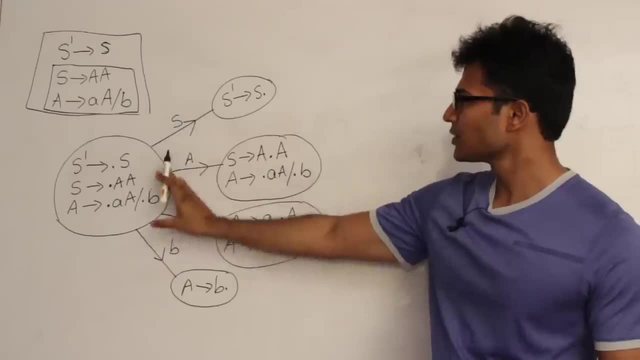 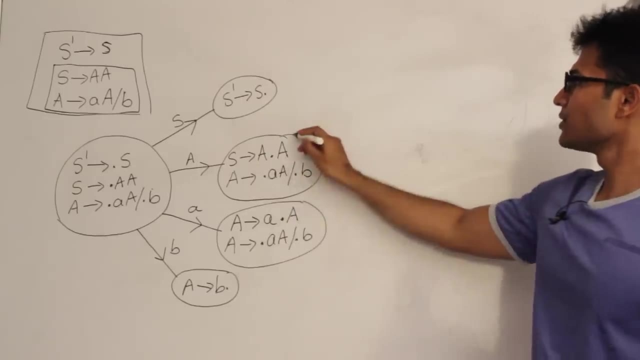 what happens on capital a. on small a, on small b, everything is complete. this one is complete. the reason is: dot is at the right hand, we cannot move it further. and this one is not complete. the reason is: dot is here, we can move it still. so, on capital a, what happens is s. 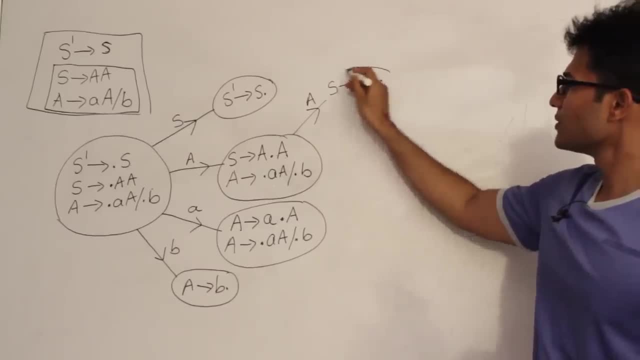 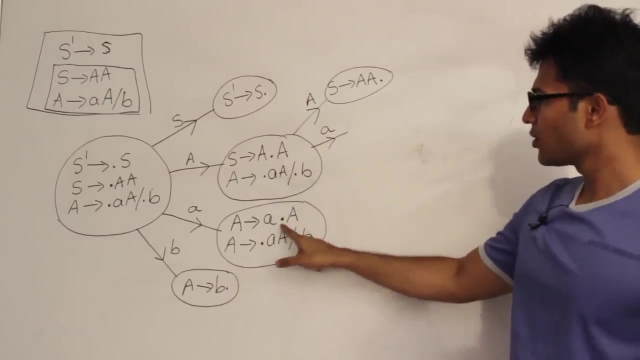 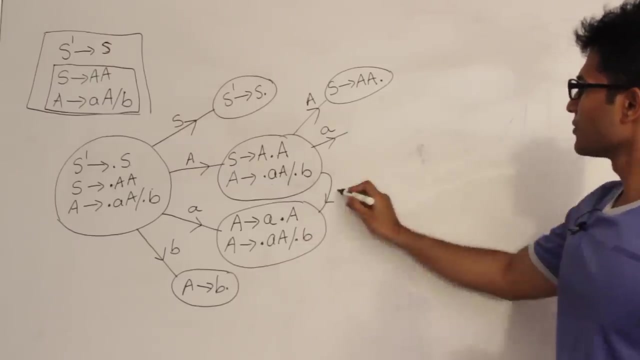 derives a a dot. this is a final item. and here, on small a, what happens is, if you see it, on small a we are going to get the same state: capital a derives small a dot, capital a, and then capital a derives a a dot b, which means on small a we are going to get the same one. 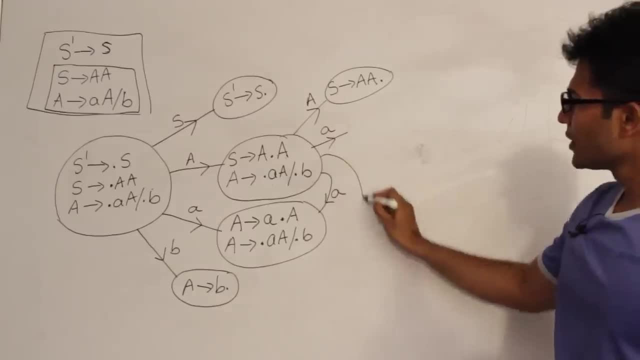 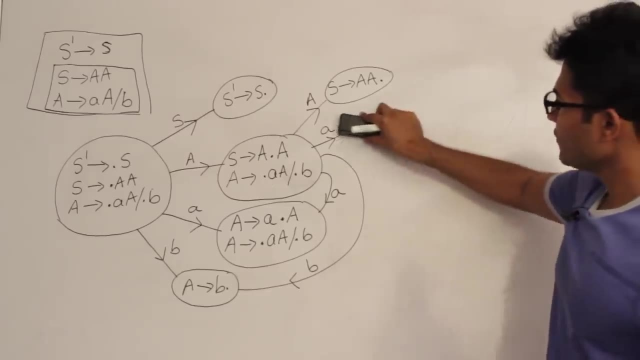 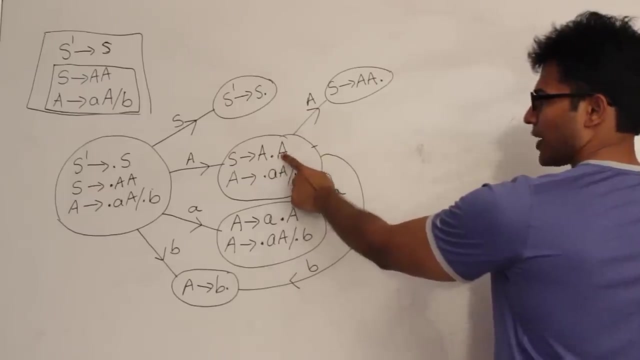 right, and on small b we are going to get the same one, isn't it? so now see if everything is over or not. so what about this? this particular state, in this particular state, we have seen what happens on capital a, we have shown what happens on small a, we have shown what happens on small b and on this, 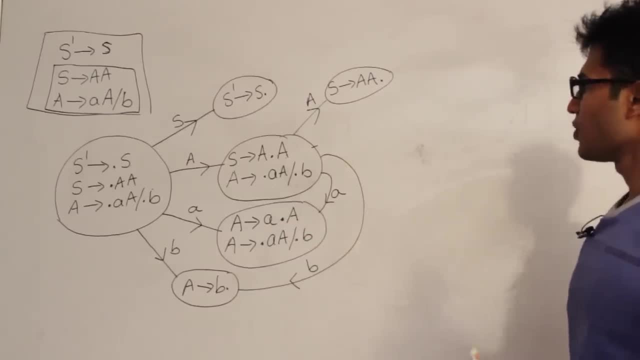 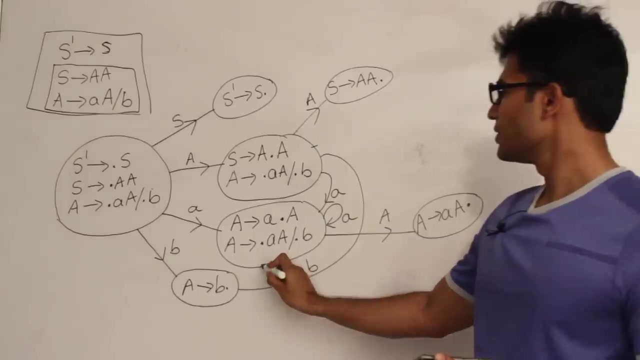 one, small a. we didn't see this right. so on small a it is going to produce the same state, and on capital a it is going to different, produce a different state. what is it? a derives, a, a dot, and on small b it is going to the same state. this one got it, so now we have shown what happens on 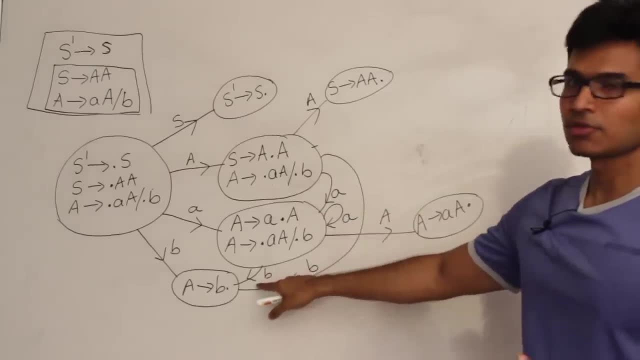 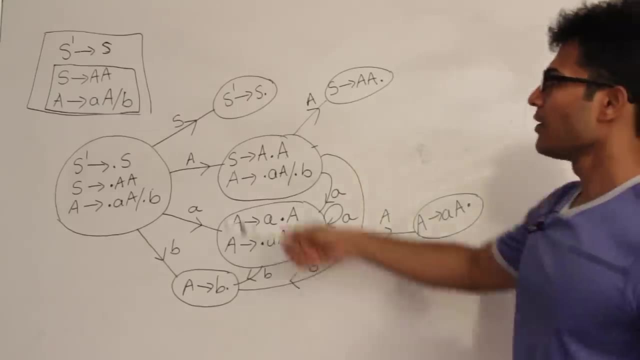 capital a. and we have shown what happens on small a and we have shown what happens on small b right. so on small b, right. so on small b right. this is the same thing, but they increase the scale. so on small b. i will show you after this. this is called canonical collection of l or 0 items. what 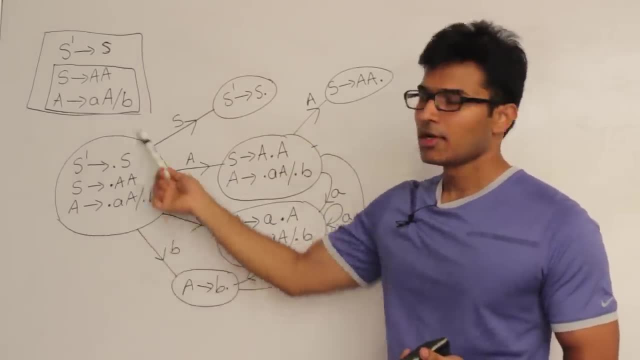 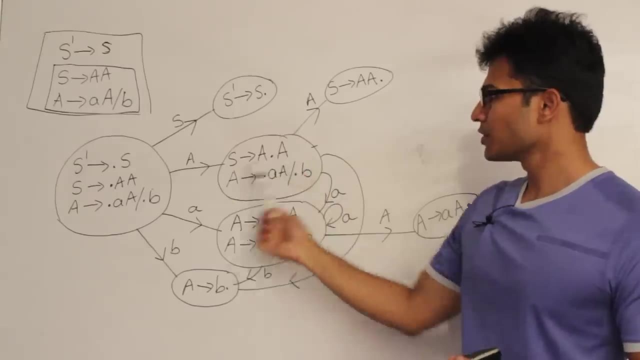 did i do? i have taken the grammar- and then i added a new production and then i started with that augmented production with dot in the beginning and i applied the closure and then i found out the transitions, which are also called as go to moves, and then again, closure go to and closure go to. 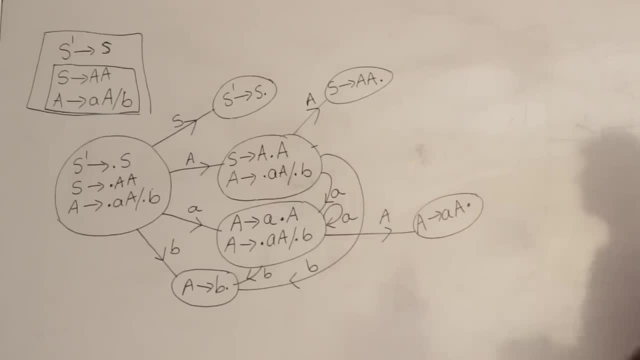 and closure. go to and closure from every state. again go to and closure. right, so i have found out What is the final item. Any item with dot at the ending is called final item. What is the importance of final item is it specifies that we have seen everything in the right hand side. 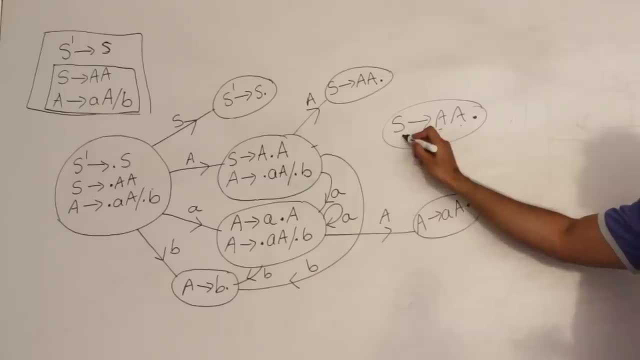 and therefore you can reduce aa to s. now We are scanning the input and now, with some part, we have seen the entire thing of right hand side and it is the time that you reduce it. So now this is called canonical collection of LR0 items. Using this, I am going to construct the LR0 parsing table. 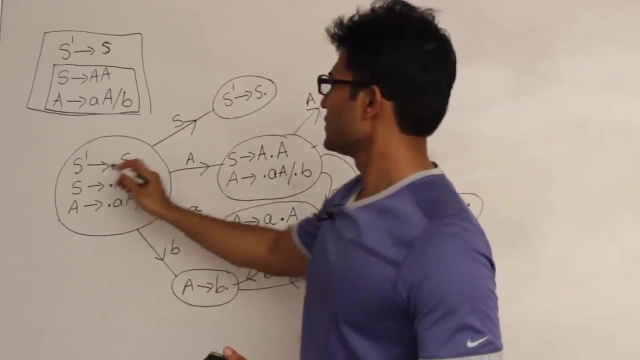 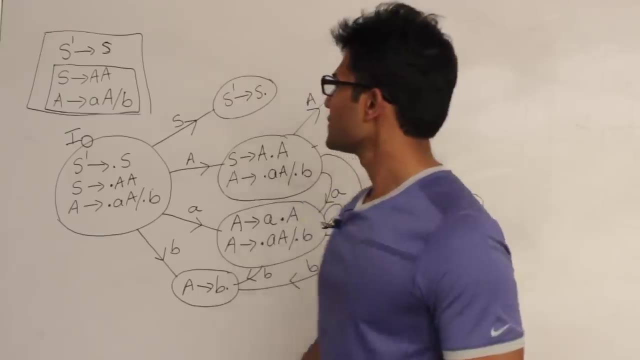 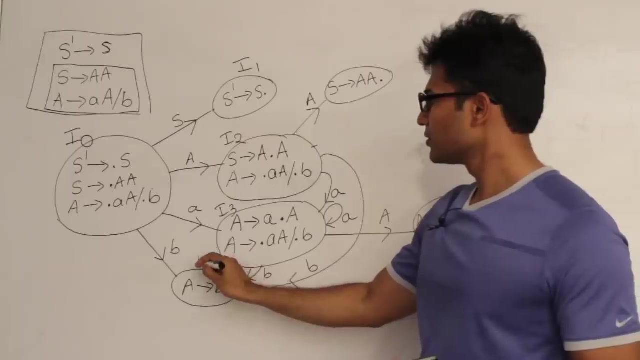 So just name the states once This state can be, for the sake of identification. I am just naming it. You can name any names here. I am calling it as I0, I1, I2, I3, I4,, I5, I6. 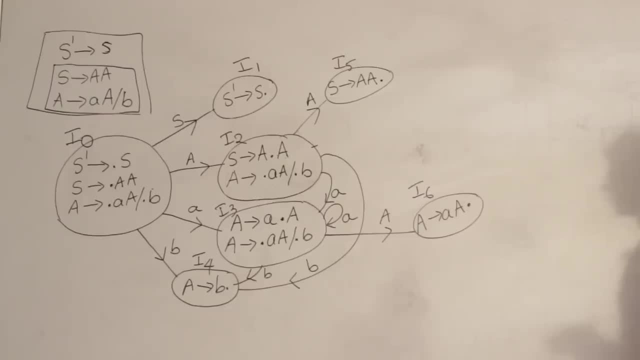 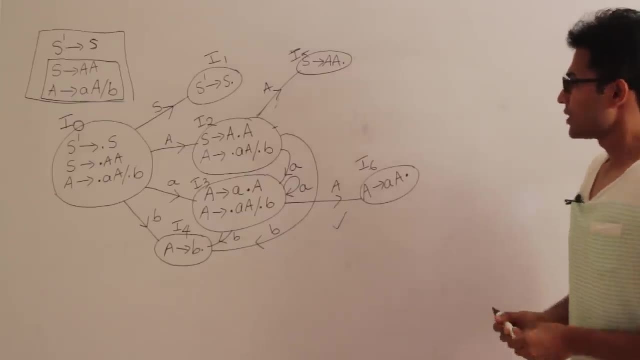 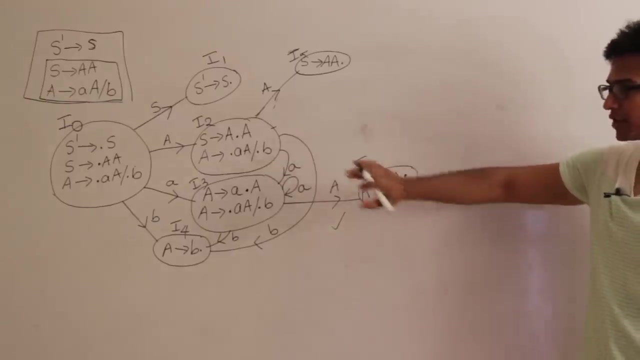 So there are totally 7 states, I0 to I6. Therefore, now I am going to construct the parsing table first For this, Let's construct the LR0 parsing table for this canonical collection of LR0 items. This is also called as canonical collection of LR0 items. 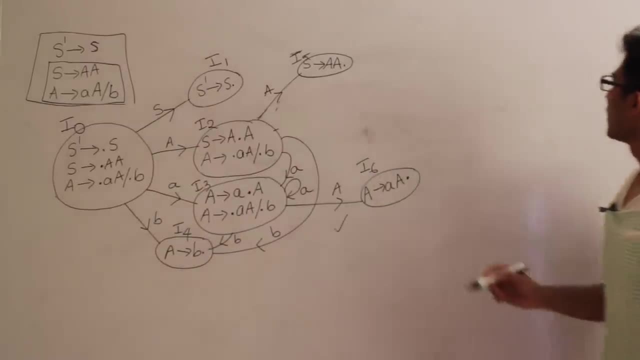 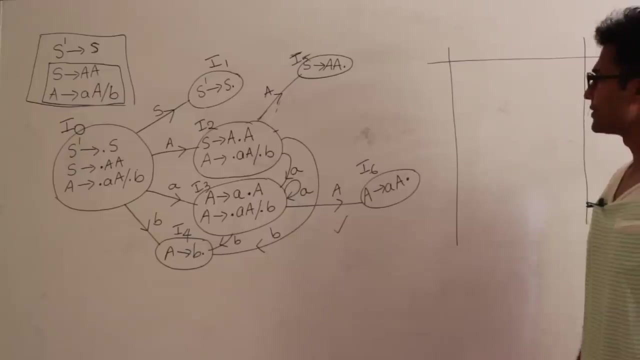 LR0 item is nothing but any production with dot in the beginning. So now, first thing is you have to see the number of states there, Number of states in the canonical collection. So we have I0 to I6, Which means 7 states. Therefore, I am writing 0, 1,, 2, 3,, 4,, 5, 6. 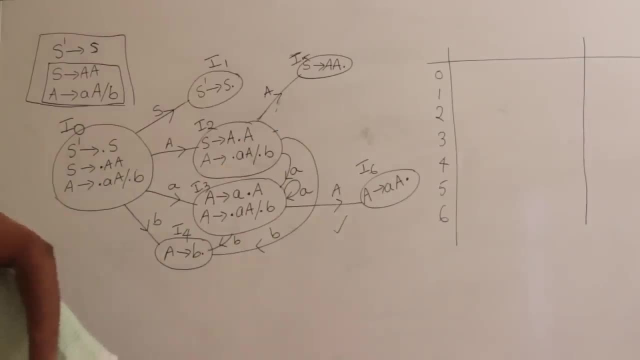 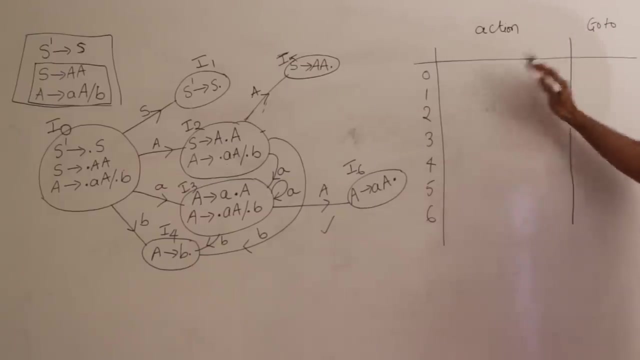 So these are all total 7 states. And now the table will have 2 parts. One is called action part, Another is called goto part. The LR parsing table will always contain 2 parts, Either it is LR0, SLR1, LLR1 or CLR1. 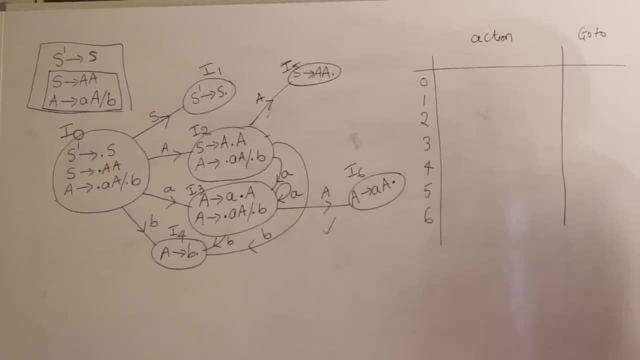 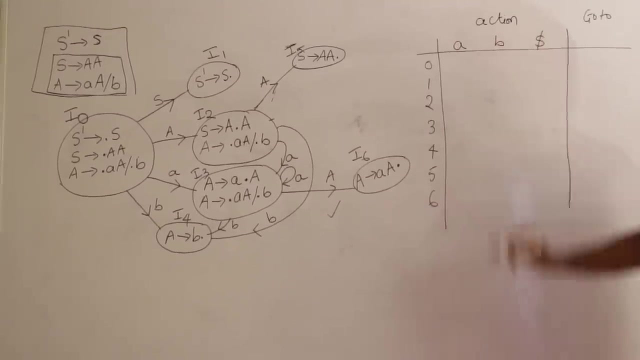 They will all contain 2 parts. Now, action part will contain only terminals. What are the terminals in the grammar? Terminals are A, B and $. These are the only terminals. And what are the goto parts? In goto part we have all the variables. What are the variables in the grammar? 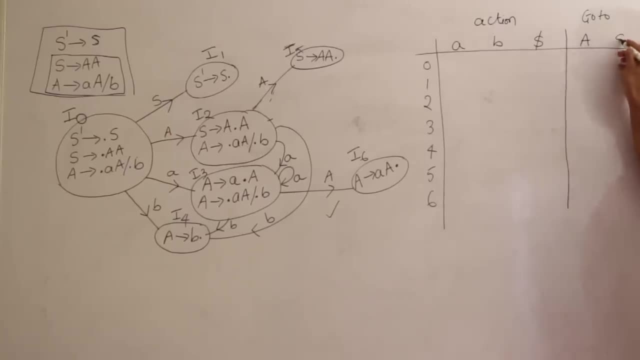 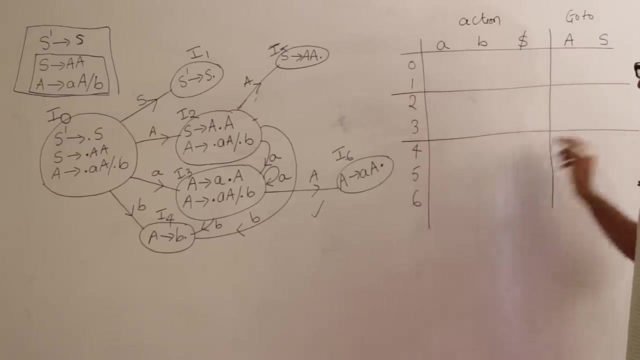 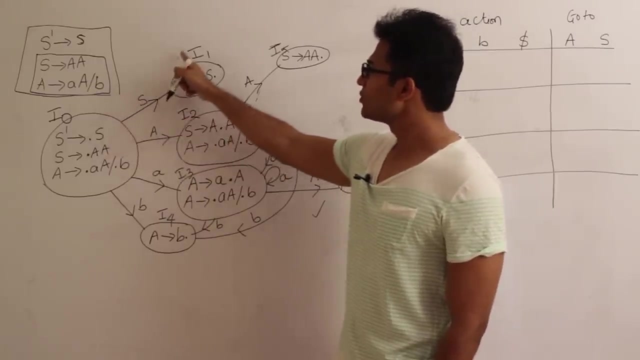 We have variables as A and S. These are the 2 variables. Now I have to fill all the entries. All the entries of all the states Now go to the state I0 In I0. on S it is going to 1. So whenever you have a transition on variables, 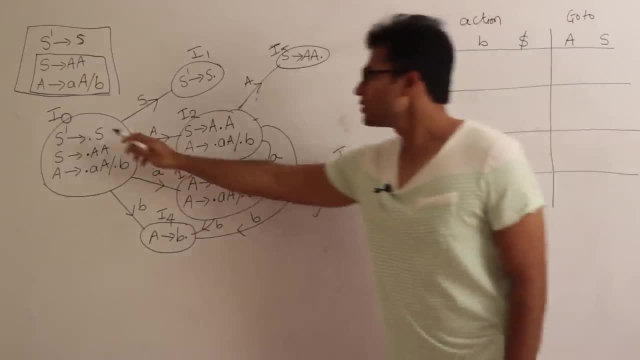 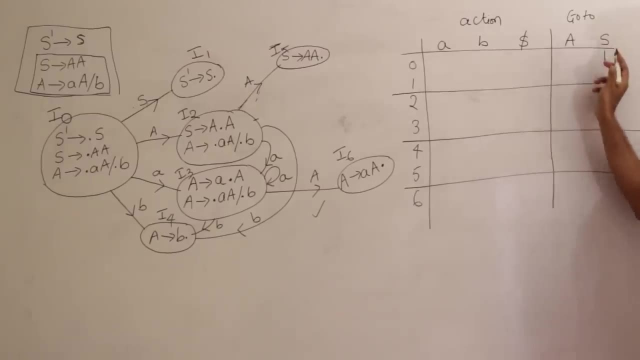 You have to go to goto part. So I0 on S is going to I1. Therefore, I am going to write it as 1, I0 on S is going to 1 And on A it is going to 2. Therefore, I0 on A is going to 2. 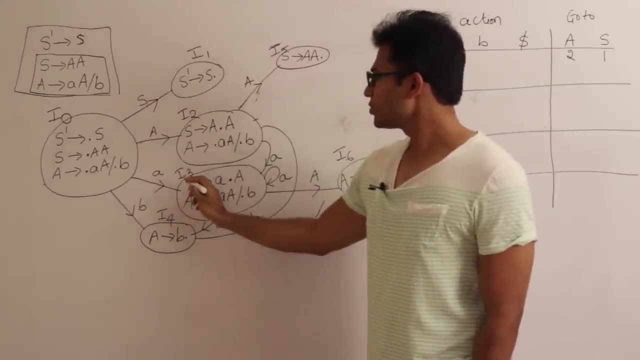 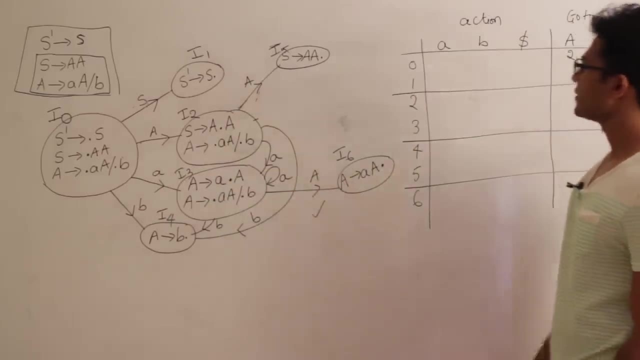 And I0 on A is going to I3. So whenever there is a move on terminals, I am going to write it as I0 on A is going to I3. Therefore, I am going to write it as S3, Which is nothing but Shift 3. 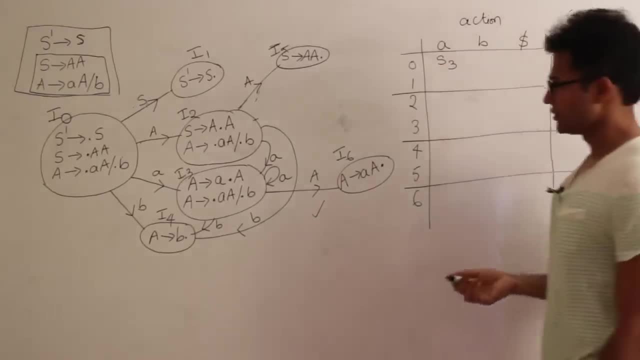 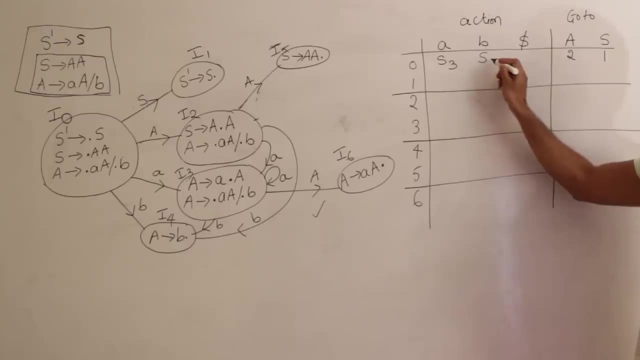 I will tell you what the meaning of it is. These are the conventions. Next one is: I0 on B is going to S3 And I0 on B is going to I4. Therefore, I am going to write it as S4. So we have 4 transitions. 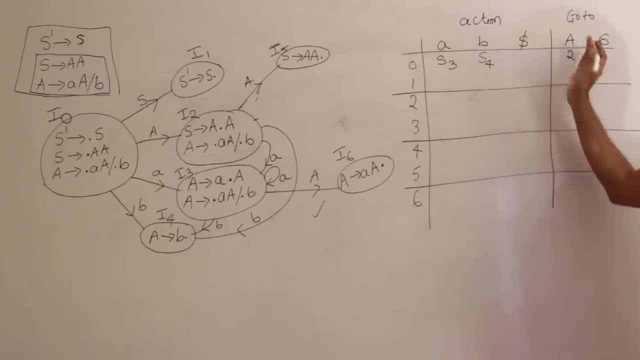 And we have 4 entries here. 2 entries are in action part And 2 entries are in goto part. Next one: let's see I2. I2 on A is going to 5 And I2 on A is going to 3, Which means S3. 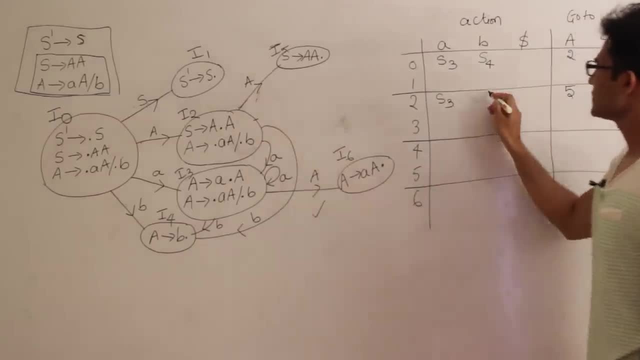 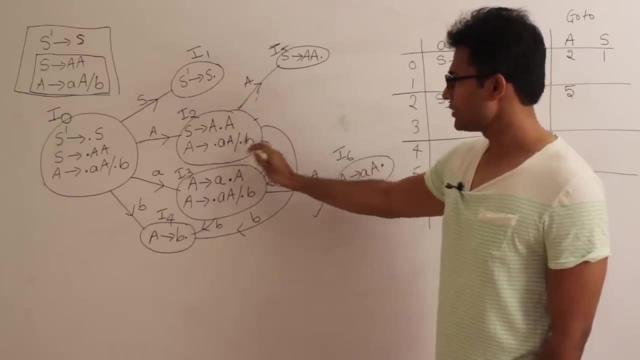 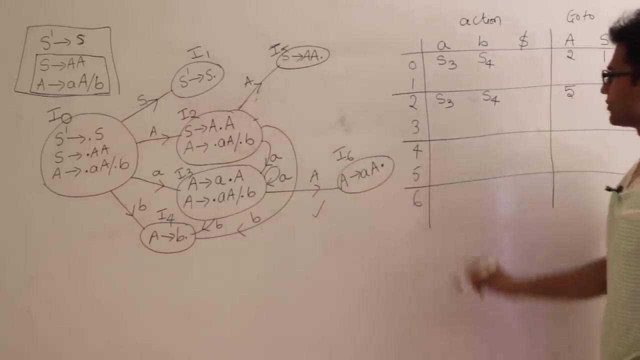 And I2 on B is going to 4, Which means S4, And that is it. We have only 3 transitions On A, A and B, Next I3. I3 on A is going to itself, Which means S3, And I3 on B is going to I4. 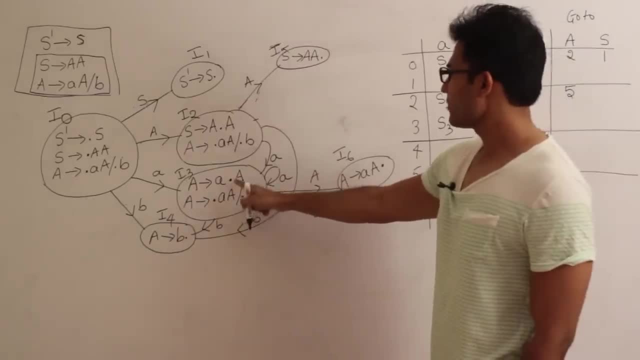 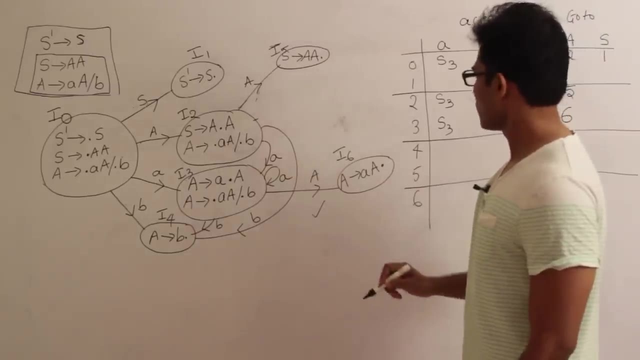 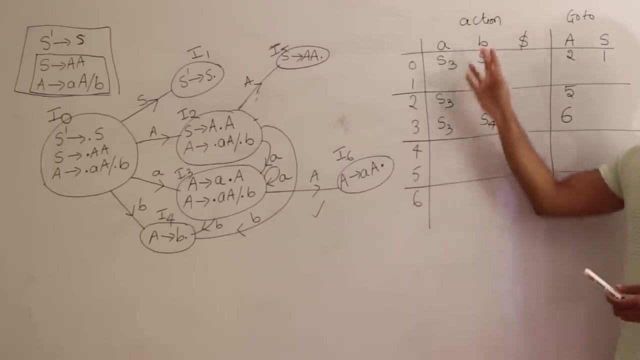 Which means S4 And I3 on A is going to 6, I3 on A is going to 6, And now we have 4,, 5, 6. So this is common for all the parsers, For all the parsing tables. Action part and goto part is common. 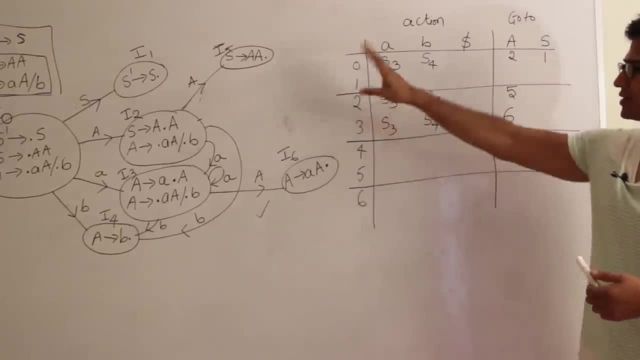 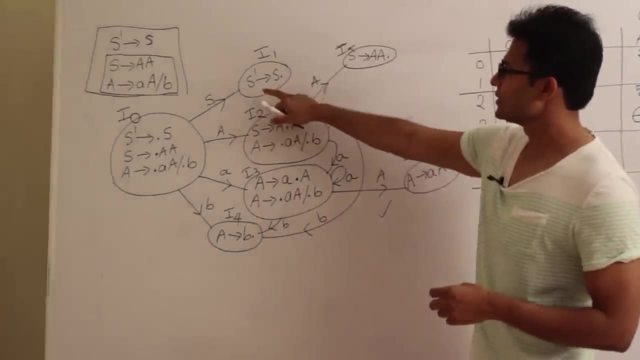 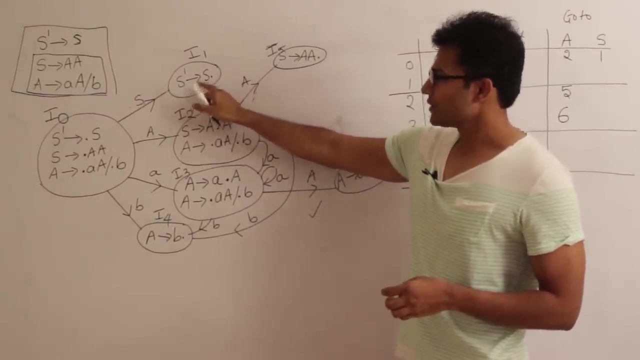 Only thing which is different is Whenever any state is having final item, Then the entries are going to be different. Now just see the state I1. The state I1 has final item Which is corresponding to the augmented production. Therefore, Only this is the exception Which is used for accepting. 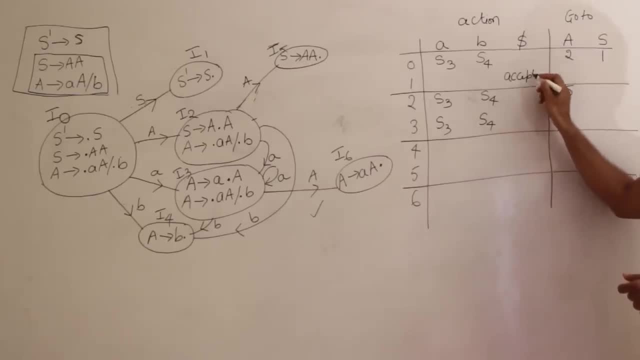 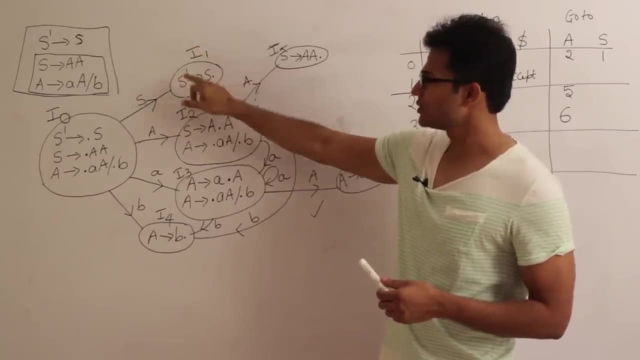 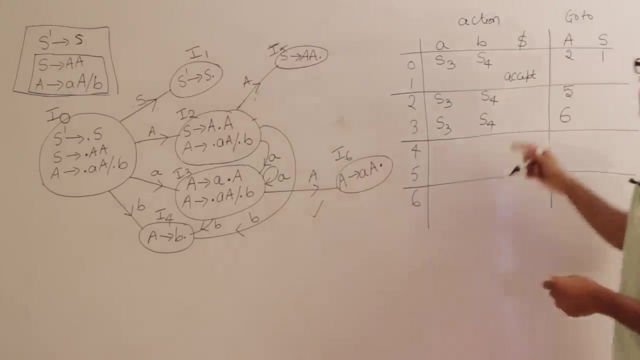 Remember it Whenever you get, Whenever you get The final production Or the final item Of the production which is augmented, We have to understand that That is a special production which is added Because we want to accept it, So we are going to accept it, Or you know the meaning of this is. 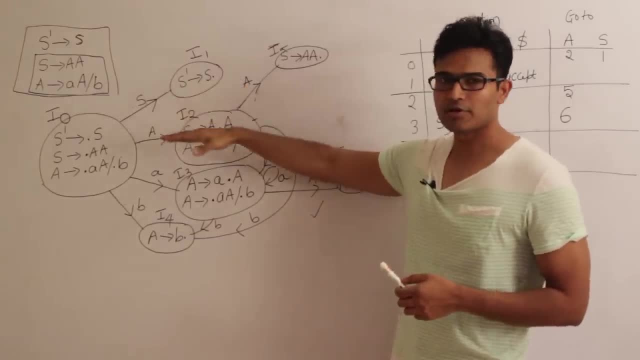 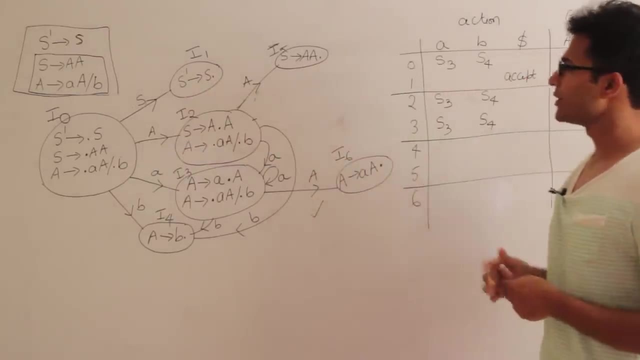 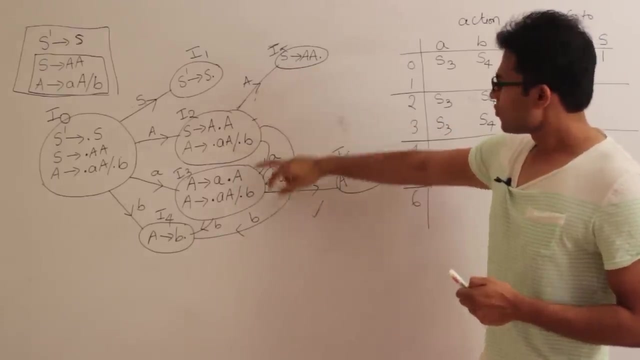 It also shows that We have seen everything of the start symbol. We started from the terminals And then we reach the start symbol. Therefore, we have seen everything. Maybe that is also a valid explanation Why we have to accept there. Next one is: Let's see I4, I4,, I5, I6. 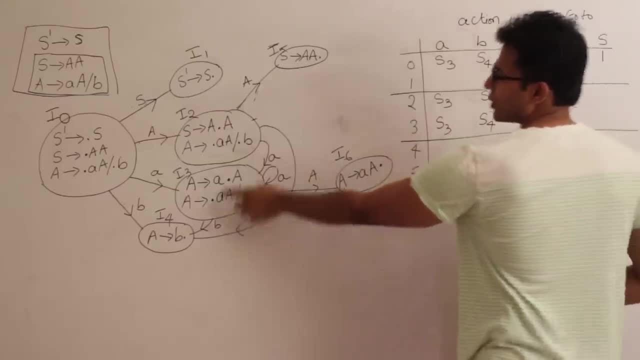 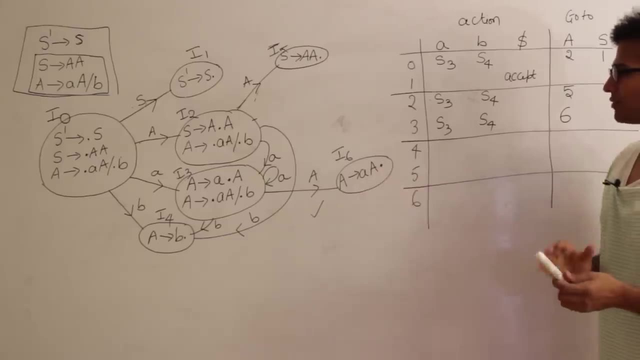 All the I4, I5, I6. I5, I4 and I6. All these states are containing the final items. Final item is any production with a dot in the right hand side, With a dot in the right hand. Write most part. Now all these final items. 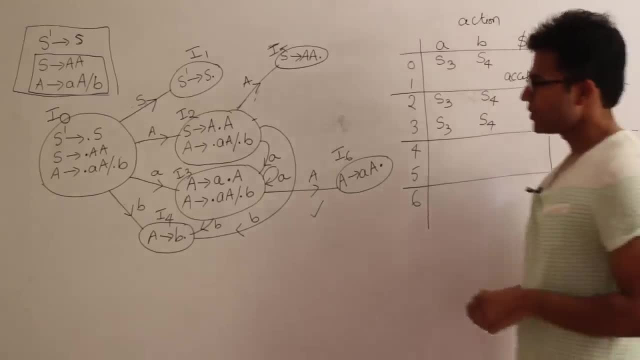 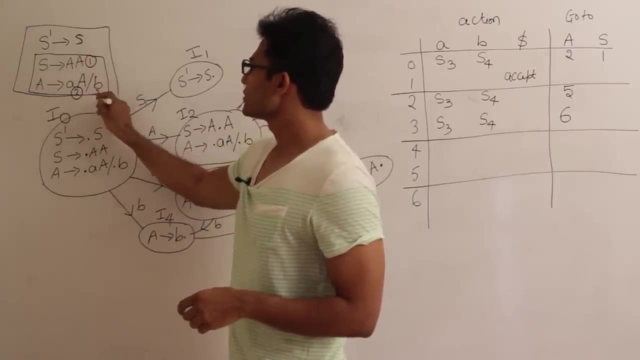 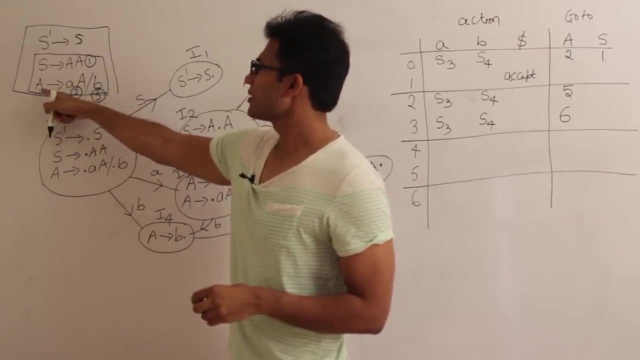 Are corresponding to some productions, Right? So let us number the productions. Let us say: This production number is 1, This production number is 2 And this production number is 3. Therefore, first production is SdAa, Second production is CdAa And CdB is third production. 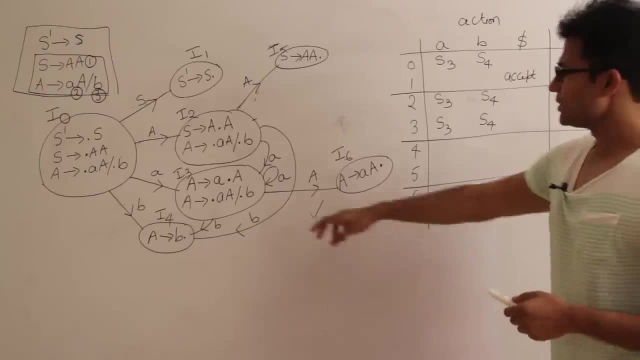 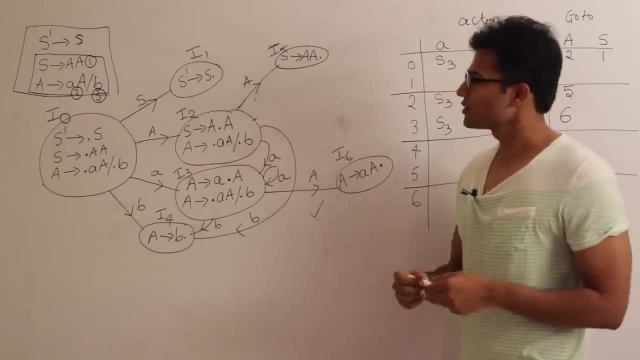 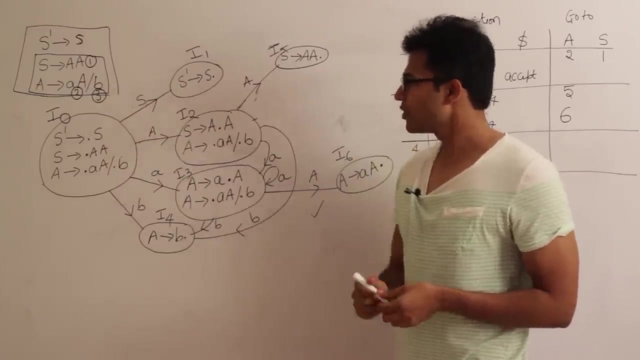 Now see the state I4. If you see the state I4, It is containing a final item, SdAa. And what is the production corresponding to this? The production is third production, Production number 3. Therefore, Therefore, For this one, The third production, I am going to write it as R3. 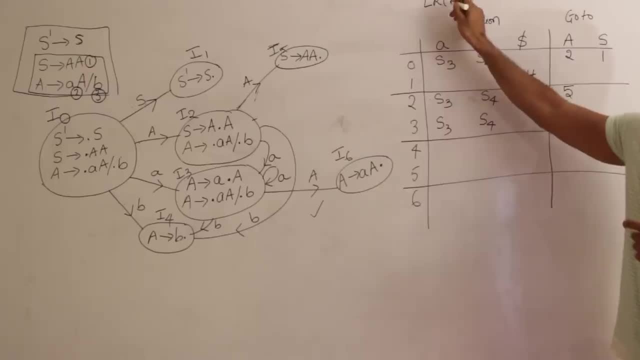 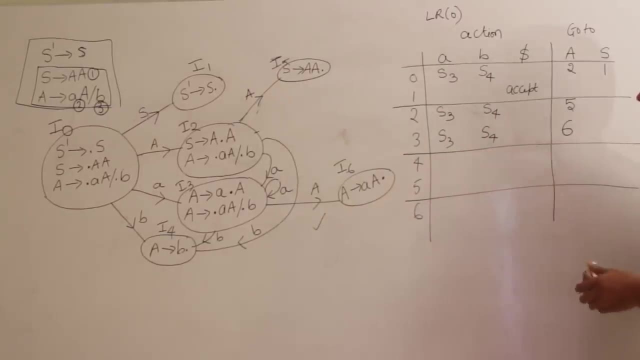 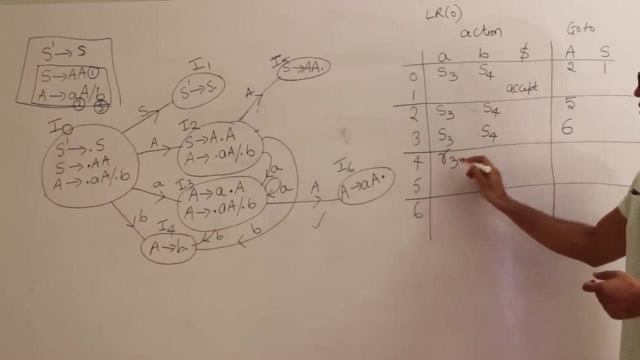 So In the construction of LR0 parsing table, Whenever any state is having a final item In that particular row, I am going to write ReduceMu completely, Which means here I am going to write ReduceMu as R3, R3, R3, R3. Why should we reduce this? 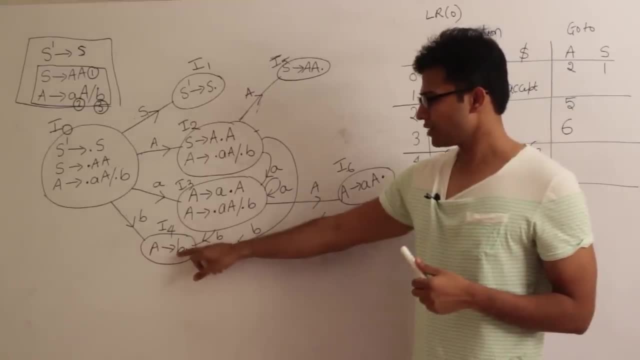 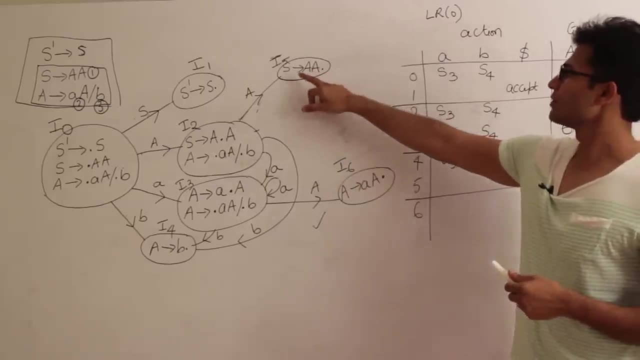 Because we have seen everything in the right hand side of a state, Right hand side of a production. Now we could reduce B to capital A. That is the meaning. And next one is: If you see I5, I5, It is also a final item And it corresponds to a ReduceMu. 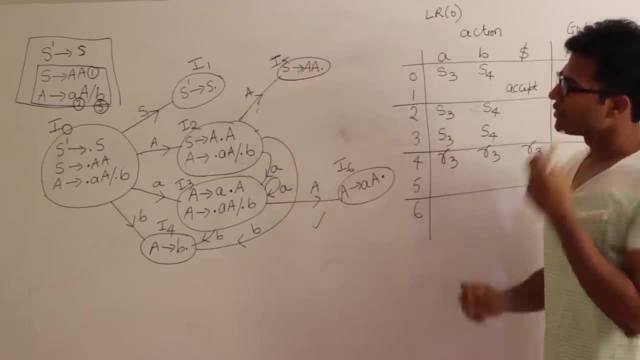 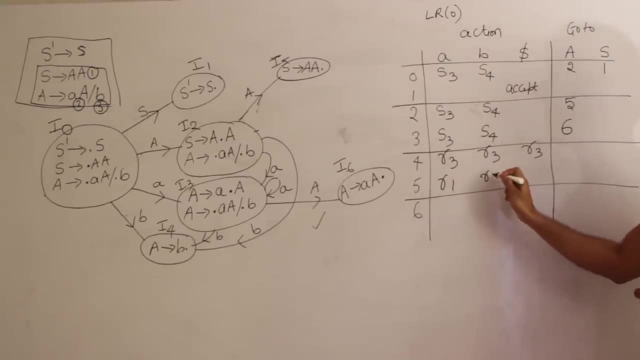 What is the ReduceMu? A is reduced to S. Therefore, what is the production number? Production number is 1, So I am going to write R1 In the entire 5th row And next one is 6th, In the 6th state. What is the production? 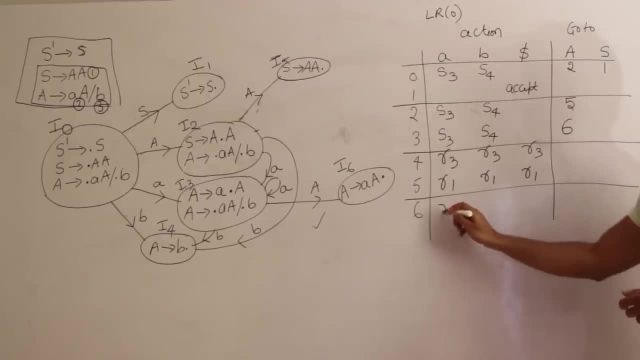 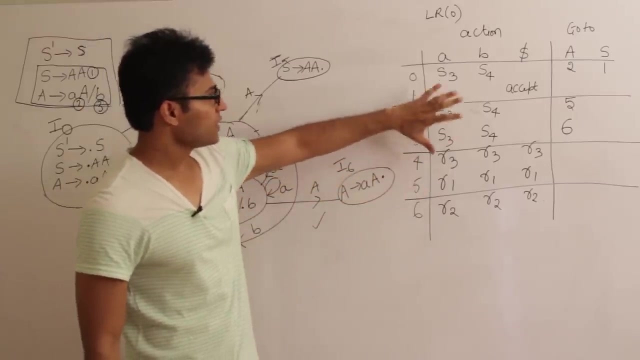 A derives AA, It is R2. I am going to write R2, So understand this How we did. it is: We have constructed the canonical collection of LR0 items And after constructing the canonical collection of LR0 items, We actually Considered all the states And we have constructed the table. 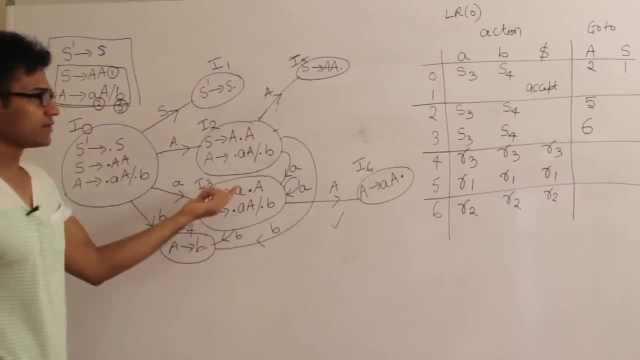 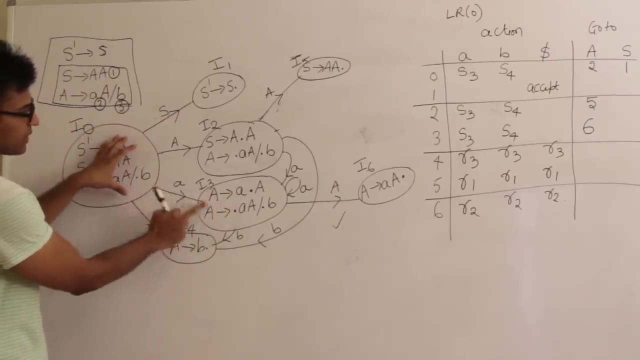 In which the number of rows is equal to number of states in this diagram. And then every ShiftMu is nothing, but Whenever there is a state And if that state is going to some other state on a terminal, That corresponds to a ShiftMu. And if a state goes to some other state on a variable. 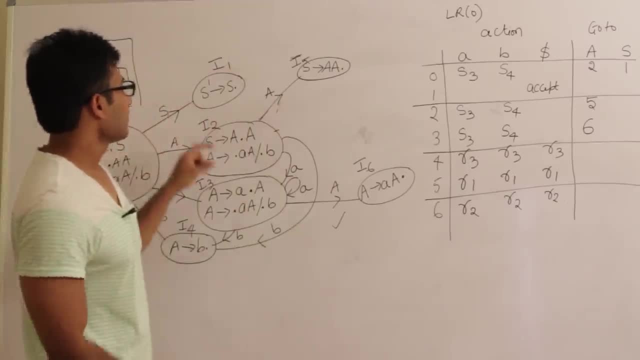 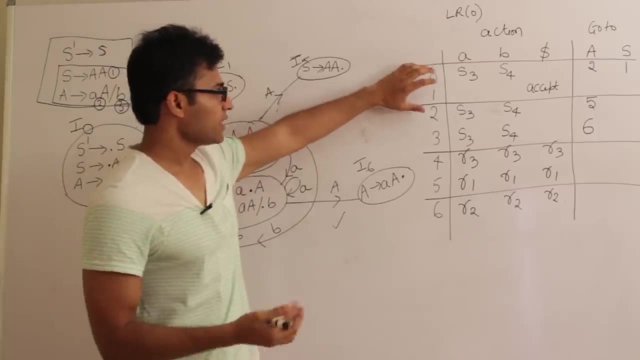 That corresponds to GoToMu. Okay, And whenever you come across this production, The production is augmented production And you have to remember that That production is being added by us. Therefore, that corresponds to the, Therefore that corresponds to the AcceptMu. And whenever you come to any state, 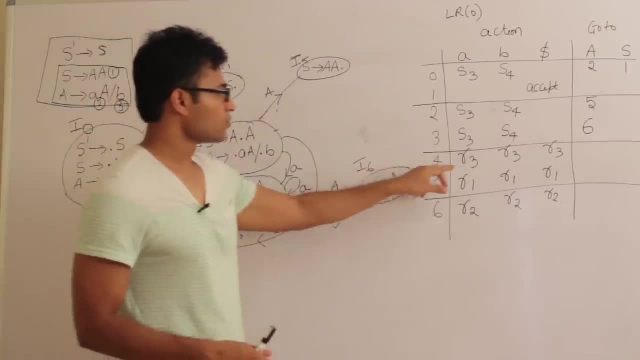 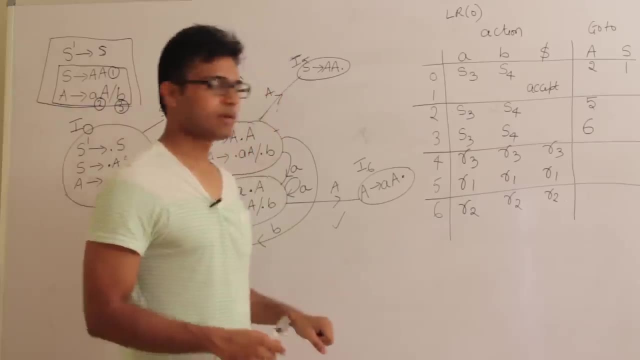 In which there is a final item, You have to write ReduceMus Of the corresponding production. For example, the production number of AA is 2. Therefore in I6 I am going to write R2. So remember this: Whenever a state is containing a final item, You have to write the corresponding ReduceMu.